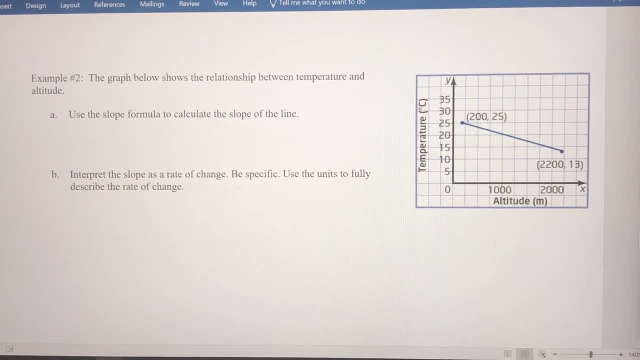 Okay, so in this video we're going to finish up those notes with a problem. where we talk about, slope is a rate of change. okay, So we introduced this concept by talking about rate of change first, and then we went over how to find slope using rise over run or using the slope formula. okay, 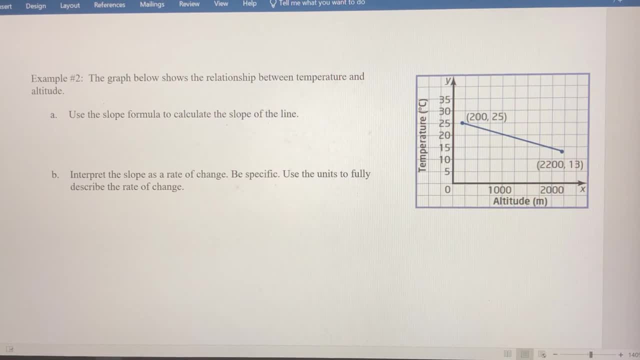 But the main thing that we have to understand is: slope is a rate of change, So those two phrases or terms are always interchangeable. If you're thinking of slope, you're thinking of rate of change. If you're thinking of rate of change, you're thinking of slope. So it's really important. 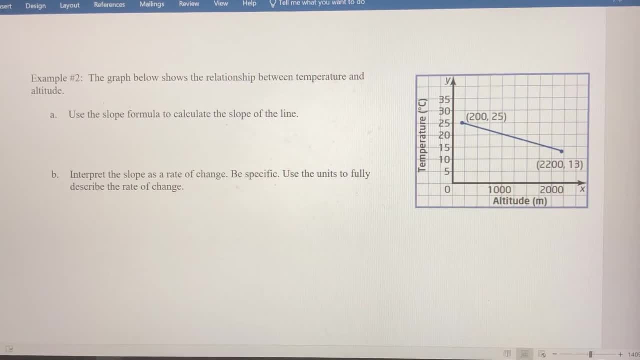 to understand the link between those two things. all right, So we've got a situation here. We've got a graph that compares temperature on the y-axis here to altitude on the x-axis. okay, And you can see that as altitude increases. okay, so as we get higher and higher and higher above. 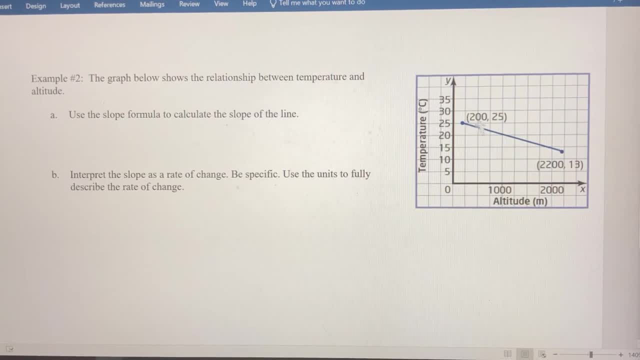 sea level. okay, then our temperature is going to be falling. okay. So just by looking at this level, we're going to be seeing that the temperature is going to be falling. So just by looking at this level, we're going to be seeing that the temperature is going to be falling. okay, So just by. 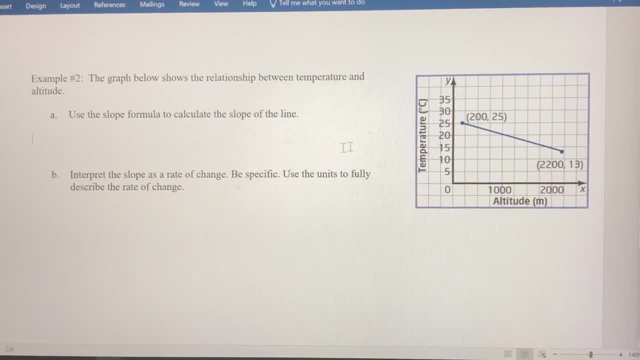 looking at this line, you should be able to tell that the slope, and because of that the rate of change, is going to be negative, because this line falls from left to right. okay, So it's always important to understand what the sign of your slope is going to be before you even start the 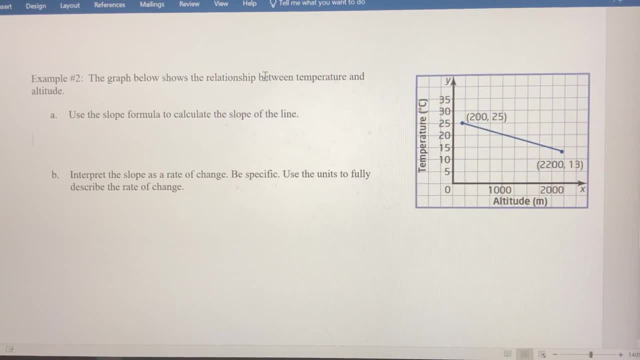 process. okay, So on the line, we know two ordered pairs- okay, So we always want to account for the ordered pairs that we know, all right, And we're going to use the slope formula, okay, to find the slope of this line and therefore we're going to be able to tell that the slope is going to be. 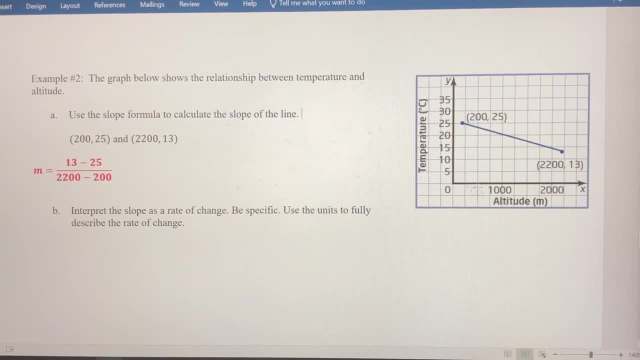 to find the rate of change of the temperature compared to the altitude. okay, So we want to subtract our y-coordinates 13 minus 25 in the numerator. In the denominator, we're going to subtract our x-coordinates 2200 minus 200,. okay, Let's simplify both. That gives us negative 12. 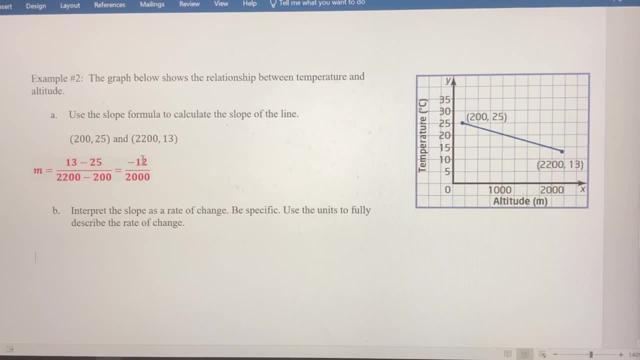 over 2000,. okay, Both these values are divisible by four. I don't want the decimal here, I want to keep this, you know, in a simplified fraction format. okay, So the most simple way to do this, we can make this fraction as negative. three over 500, okay, The decimal representation of this.